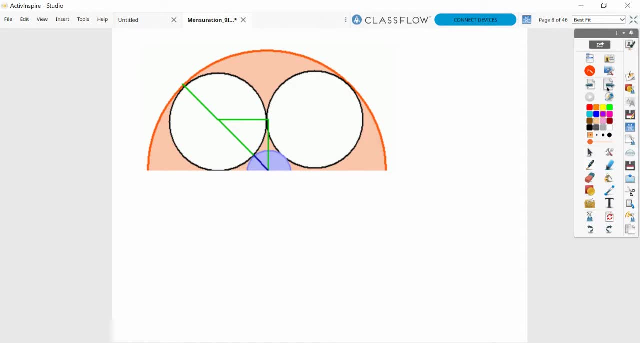 like. So we are just bothered about this figure. Now, the white, orange and blue circles are connected. Let us take the radius of the white circle as x. So if this is x, this is also x. This is the radius, And let the radius of the blue circle be y. So one connection that we have. 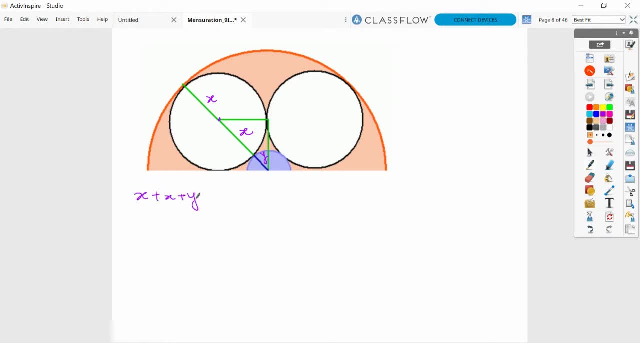 between x and y is that x plus x plus y is equals to 10, because this is the radius of the large circle. So 2x plus y is equals to 10.. This is a linear equation and two variables. We need one more such equation. 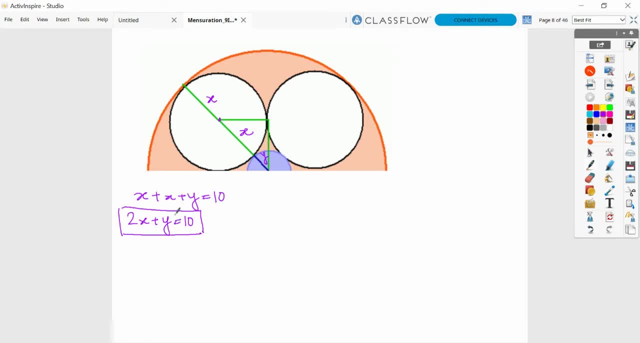 so that simultaneously we are able to solve these two equations. So here we are trying to connect the dots and we have joined the point of contact between these two circles and the center of the smallest circle here. So we join this, we join this. 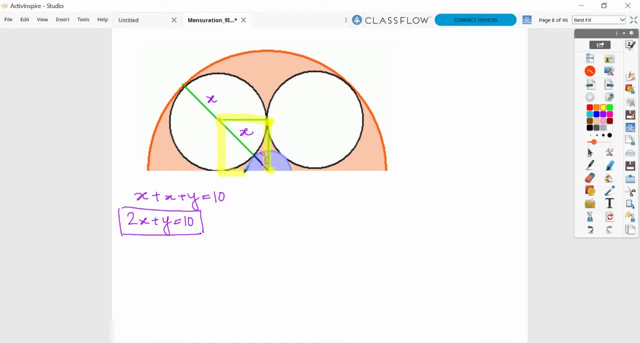 They will be perpendicular and this ultimately will be a square. So we also have a connection between the diagonal of a square and the side. So if this is x, this is also x, Right. So can we also connect that x plus y is the diagonal of this yellow square. 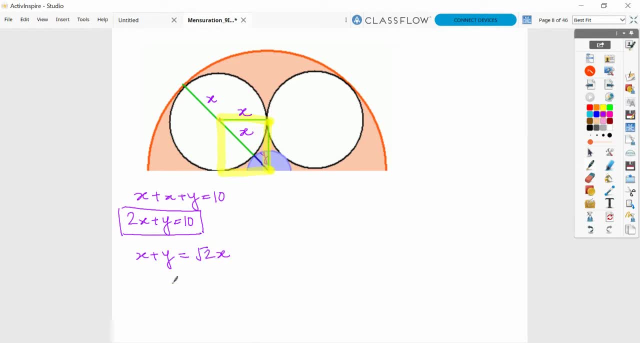 which is actually root 2 of the side of the square, That's x. So root 2 x minus x equals to y. This is another equation that we can use to solve Now. we can solve them by eliminating y, or we can use substitution method to solve these two simultaneous linear equations. 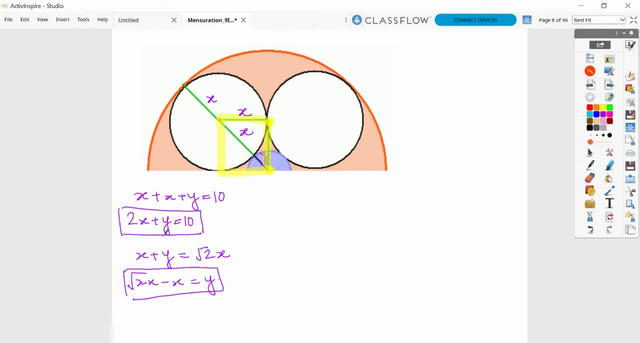 Let's substitute the value. Let's substitute the value of x, so that we can directly obtain y, which is our objective. So we take root 2 minus 1 here and x common. So x equals to y upon root 2 minus 1.. 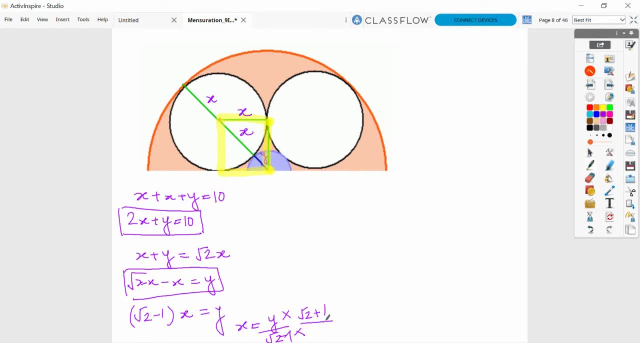 I'll try to rationalize it so that it becomes simpler to handle. I multiply both the numerator and denominator with root 2 plus 1.. So this is root 2 plus 1 times y. I multiply both the numerator and denominator with root 2 plus 1 times y. 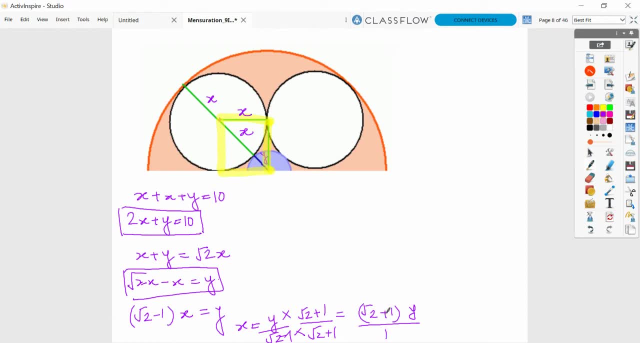 Upon 2 minus 1, which is simply 1.. Let's now substitute this value of x into the first equation, so that we'll get a linear equation in one variable. We could have also used Pythagoras theorem to connect them. That will give you a quadratic equation.